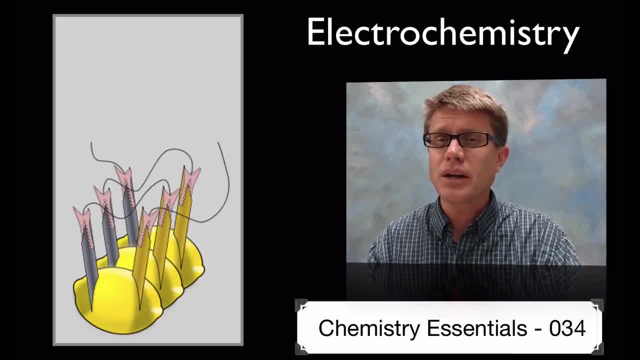 a redox reaction is. you may want to look at that video, But a great example of electrochemistry could be a lemon battery. All we're doing is inserting two pieces of metal into the lemon and we're going to generate voltage. Now you'd have to hook it up to a pretty sensitive 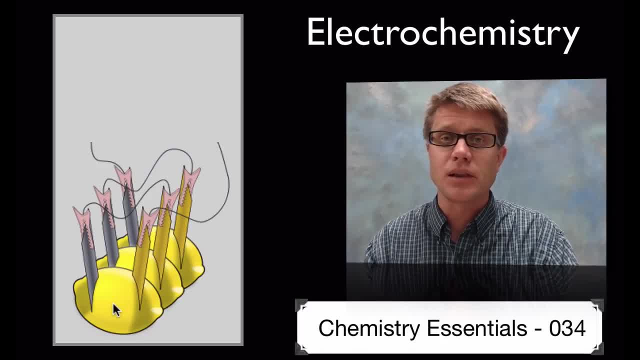 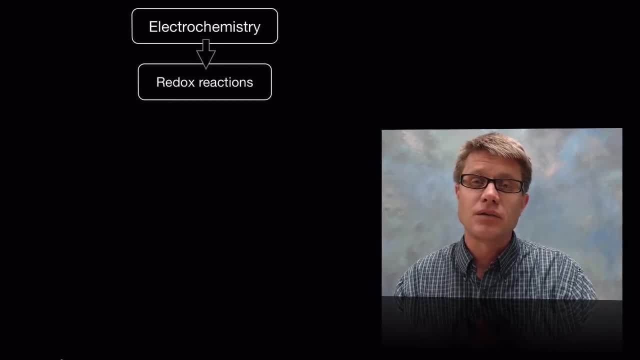 voltmeter to measure that voltage, But if we hook a number of lemon batteries up in series, we could actually light a little LED, And so electrochemistry is really the study of redox reactions, And we're separating the reduction and the oxidation portion in space. 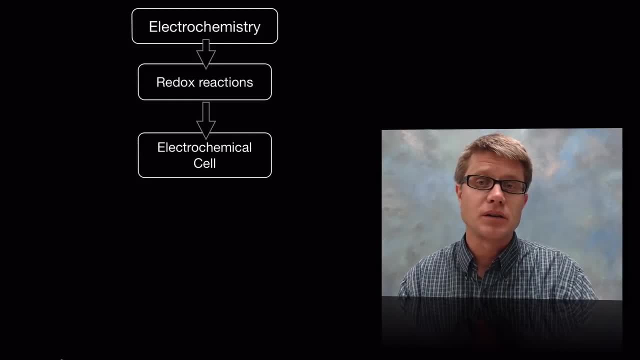 or time. Now, when you do that properly, you've created something called an electrochemical cell. That cell could either be a galvanic cell- It's sometimes also referred to as a voltaic cell. An example could be a battery And that's going to generate current Or we. 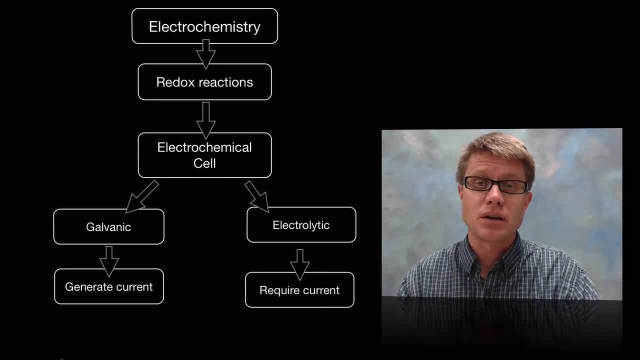 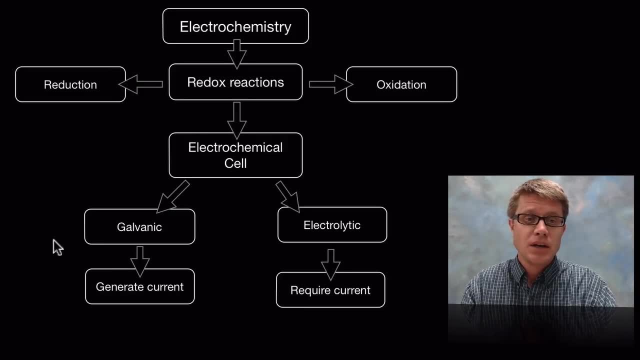 could have an electrolytic cell, and that's going to require current. An example could be a rechargeable battery. And so what we're doing, remember, is separating the reduction and the oxidation. In review, reduction is the gaining of electrons and oxidation is the losing of those electrons, And what we're doing is tapping the flow of those electrons. 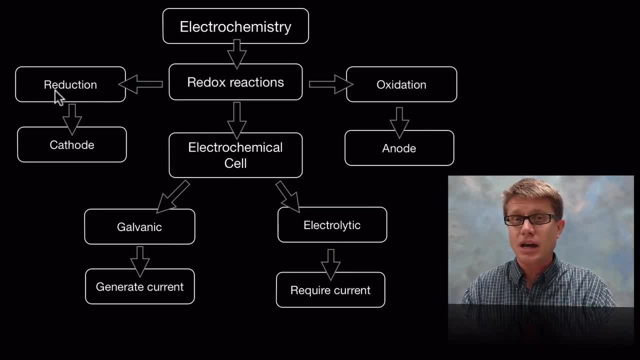 Now the metal is either a cathode or an anode, And a quick way to remember that is, the reduction always occurs at the cathode and oxidation at the anode. Or a better way to remember that is that the consonants R and C are going to pair And the vowels the O and the A are. 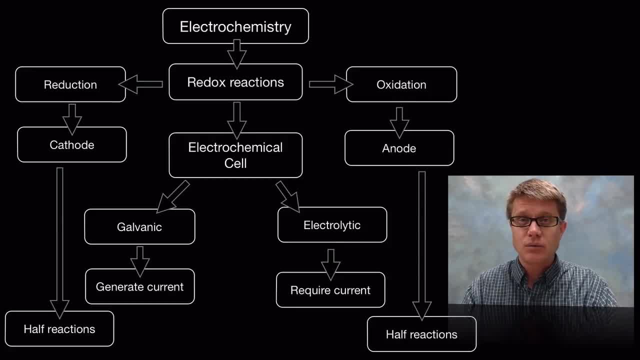 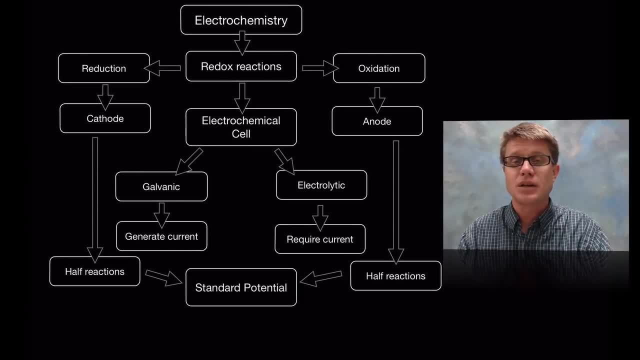 going to pair as well, And so what we can do is analyze this cell. We can break it down into its two half reactions. We could figure out the potential of those two half reactions and then simply add them together to figure out the standard potential, So how much energy that cell could produce or require if it's electrolytic. 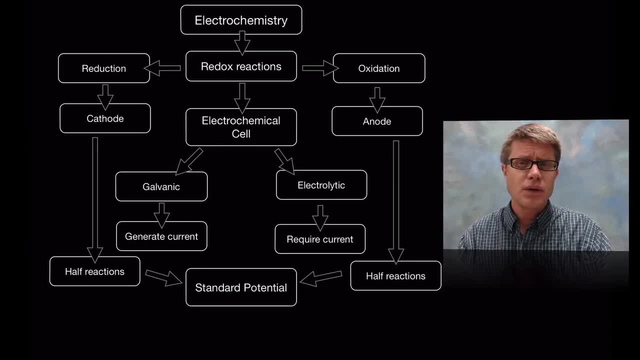 Now this would be at STP standard temperature and pressure, And so if we have variance from that, then we could use Le Chatelier's principle to qualitatively measure what's going on. We can also measure stoichiometry in a cell, So we could use Faraday's laws to qualitative. 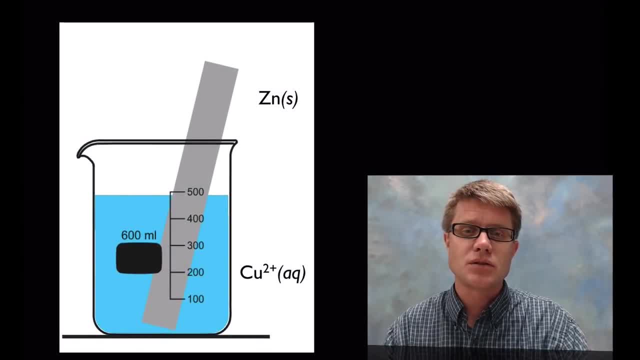 measure that as well, And so let's start with a simple demonstration. Let's say we take zinc solid and we immerse it in a copper solution. What will happen over time is we're going to get a reaction, And what you're going to 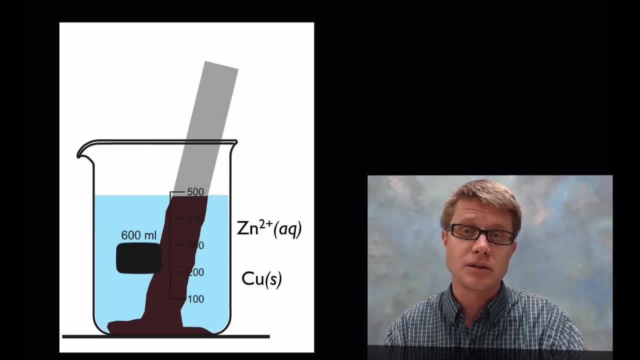 find is that zinc is going to start to become an ion dissolved in the solution and the copper is going to start to form a solid. So you'll actually form this solid copper on the outside, And so that's a redox reaction. It's reduction, It's oxidation, There's electrons flowing. 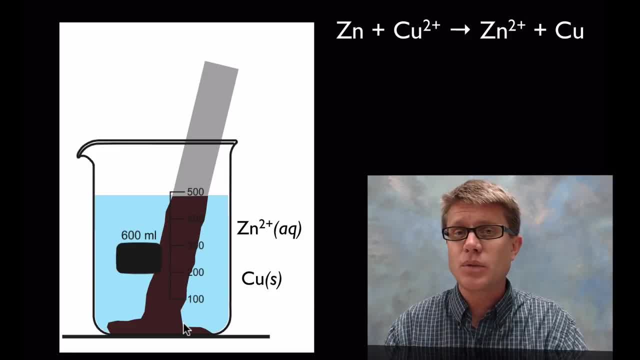 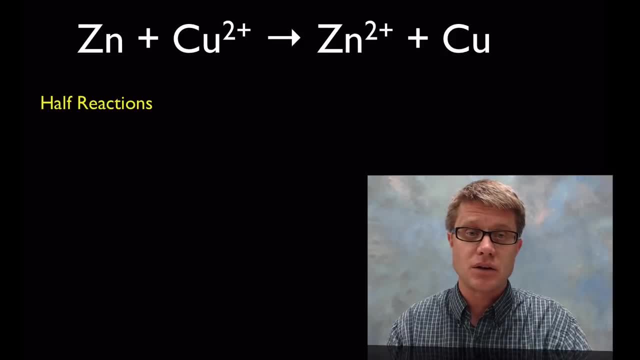 there, but we're not tapping any of those electrons, And so this would be that whole redox reaction. Again, we have the zinc which is losing those electrons, and the copper which is gaining those electrons, And so if we break it down into its two half reactions, it's going to look like this: Oxidation. 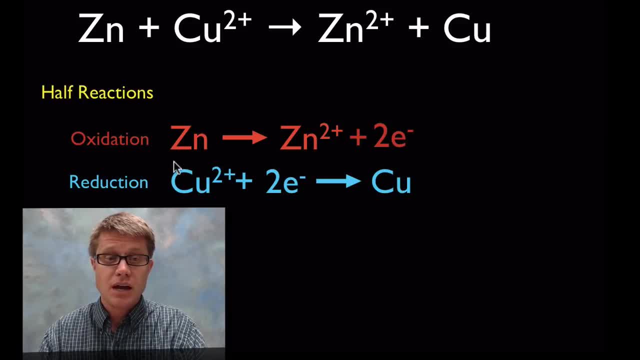 is where the zinc is losing its electrons and the copper is gaining those electrons. Those are the two parts, And so in a cell, what we try to do is separate those. But before I actually show you the cell, I want to talk about the reduction potential, In other words. 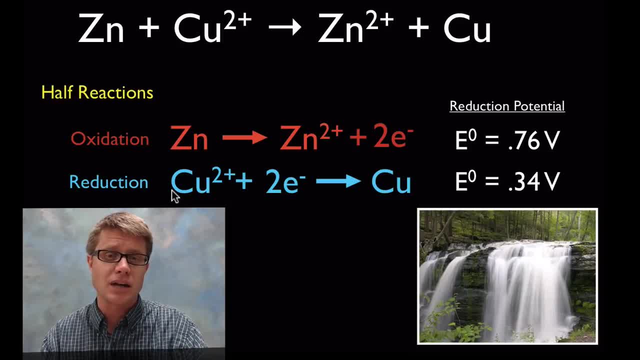 that's the potential energy that can really be released in a reaction like this, And so the zinc being oxidized is like a waterfall, In other words, it has energy up here and it's releasing that energy, And we can measure it as 0.76 volts, And so you could look up standard reduction potentials and you'll find. 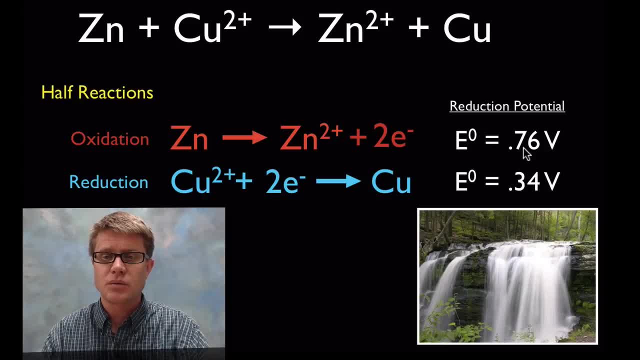 a list of these for a number of different reduction and oxidation reactions. Now the cool thing is, if we run it in the other direction, then it would be negative 7.6 volts. In other words, it would be like trying to move the water up again. We require that energy, So 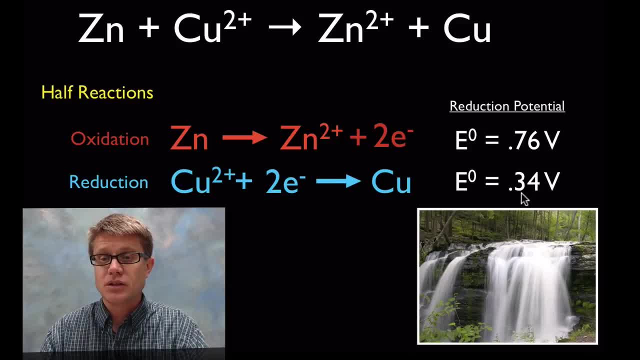 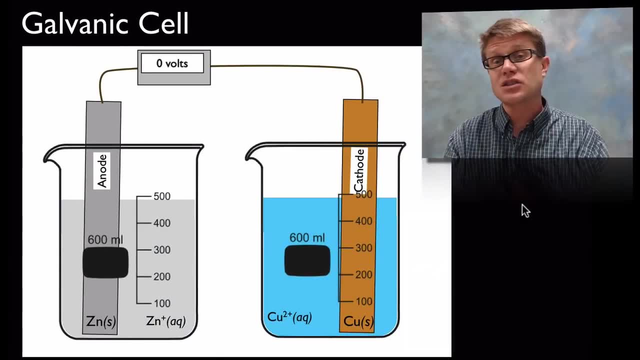 we look at the reduction part, this copper gaining of electrons, it's going to have a reduction potential or an E0 of 0.34 volts. Okay, Now let's actually build that cell, Let's separate the reduction and the oxidation portion, And so over here we have the anode. 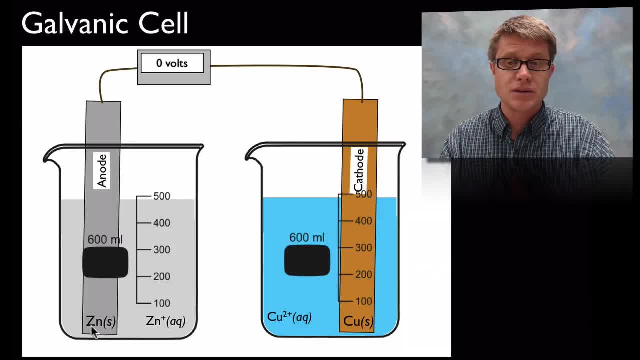 That's going to be where that oxidation takes place, That oxidation of the zinc, And then we have the cathode And they're each going to be in a different solution. So right here we've got copper metal in a copper solution, And then over here we have zinc ions in a 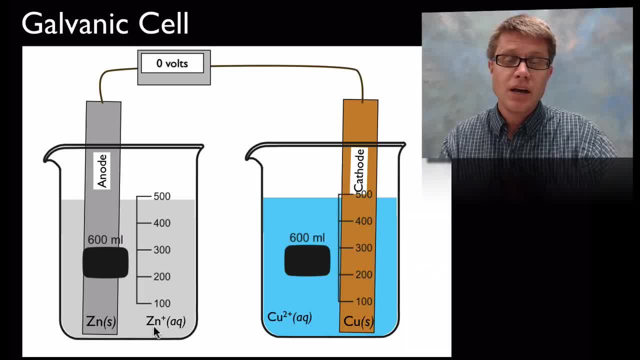 zinc or, excuse me, zinc solid in a zinc solution, And if we just let it sit like this, nothing will happen. In other words, it's not going to generate any voltage if we add a little volt meter here up at the top, And the reason why is that we haven't completed the circuit. 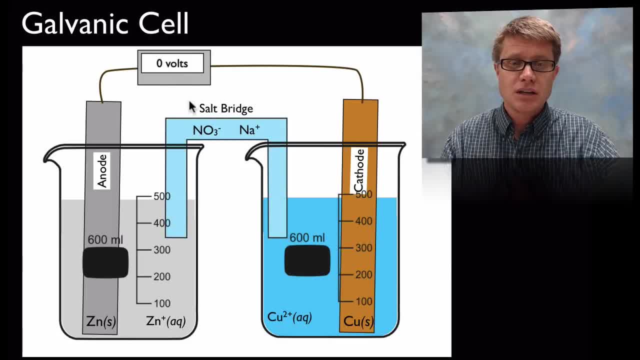 And so to do that, we're actually going to have to add a salt bridge. A salt bridge is going to be filled lots of times with a gel- In this case, we've got sodium nitrate- And what it's going to do is it's going to allow the ions to actually flow. So once we've added, 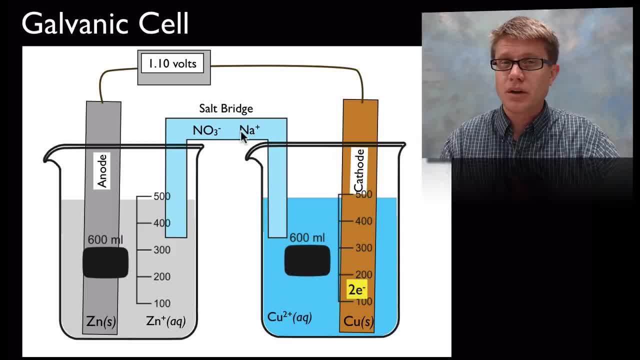 the salt bridge. this thing is going to turn on And electrons are going to flow from the anode to the cathode. In other words, the electrons that are being lost in this zinc metal as the zinc becomes a zinc ion are going to travel through the wire to the cathode, where they're. 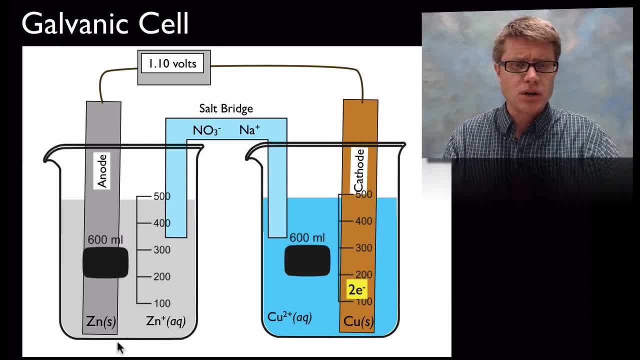 going to actually pick up those electrons. And so let's talk about what's going on over here in the anode. This zinc metal, this zinc solid, is actually moving And it's actually moving off into an ion in the solution itself. As it does that, it's losing those electrons. 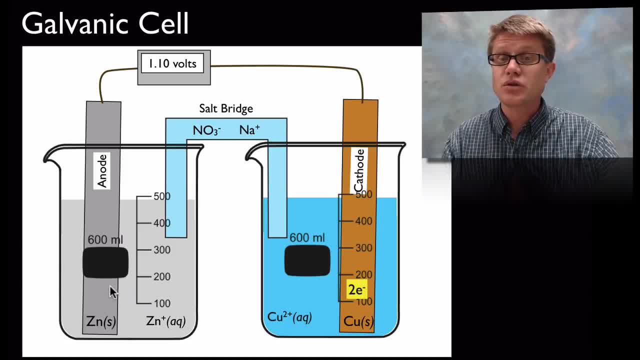 And so it's also losing mass. In other words, this anode is going to lose mass over time. If we look over on the other side, the cathode is actually going to gain mass Because that copper that's in solution is going to combine with those electrons that are coming over. 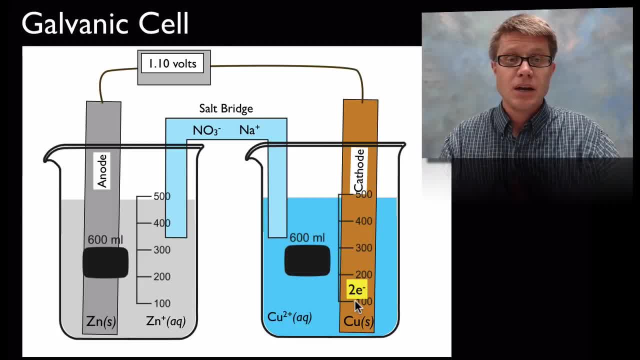 from the anode And it's going to form a copper metal, And so we can see that the voltage is 1.1 volts. How did I get that 1.1 volts? I simply added up But the reduction potential of those two half reactions. Now, how long is this going? 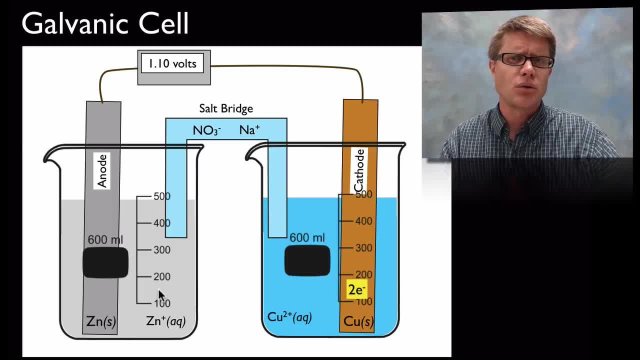 to occur. It's going to occur until it reaches some kind of an equilibrium, And so it won't last forever. Now there's an Ernst equation you could use to analyze what happens if it's not really at standard potential. But that's outside the level of AP chemistry. What you 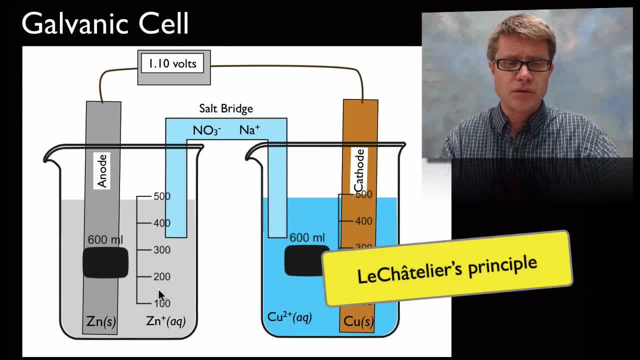 should really use is Le Chatelier's principle. So what would happen, for example, if we increase the amount of zinc on this solution? That would slow this reaction. Or if we were to increase the amount of copper- It's going to reduce the amount of zinc, So we would slow this reaction. Or if we were to increase the amount of copper. 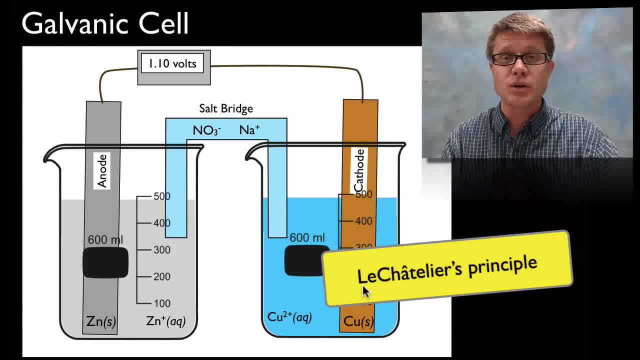 It's going to speed up this reaction. What happens if we increase the temperature? That's going to speed up the chemistry. It's going to speed up this reaction and it's going to be quicker. In other words, we're going to generate more volts than we would if it was. 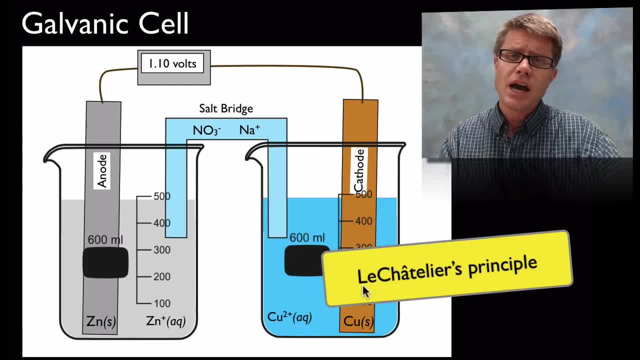 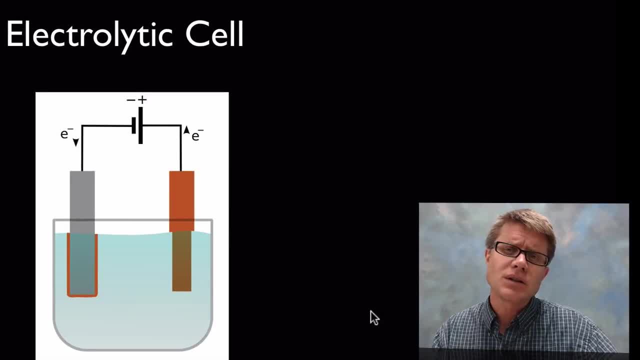 at a cold temperature. And so you should qualitatively kind of understand how a chemical reaction or things that would affect a chemical reaction could convert to things that would affect this cell. Now, what's an electrolytic cell? It's really essentially the opposite of that. 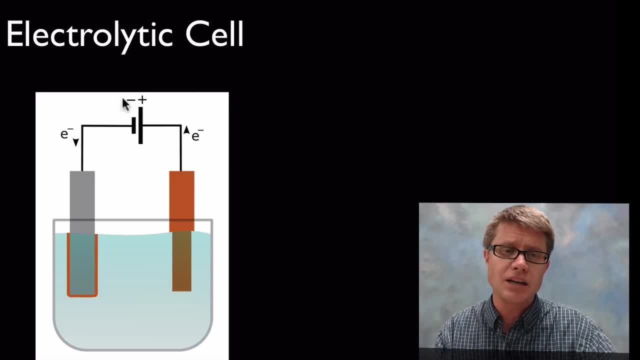 In this one, what we're going to do is add current. In this case, we're adding a battery on this side and we're actually going to cause electrons to flow. A great example of this could be electroplating, when we're actually adding one metal to the other side, Another. 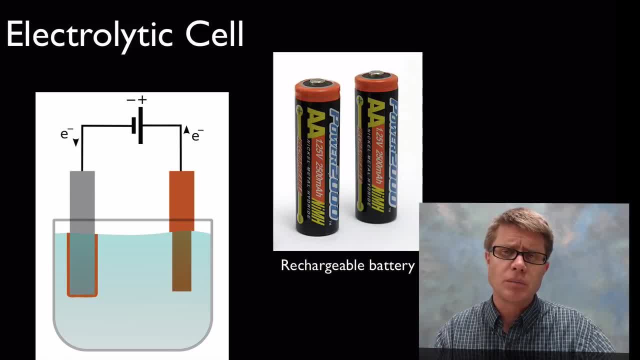 example could be rechargeable batteries, And so the way a rechargeable battery works is you hook it up to electricity And what it does is it acts as an electrolytic cell. It's going to store energy inside the cell. Now you unplug it from electricity and now it. 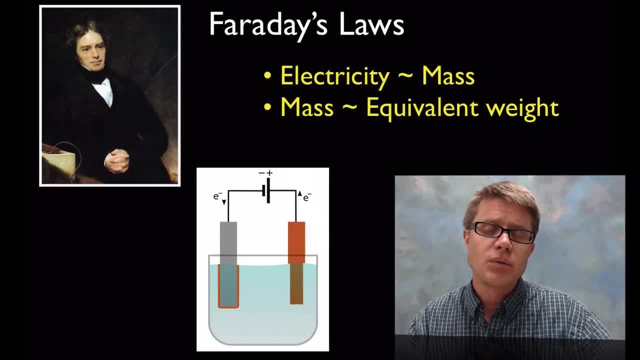 becomes a galvanic cell, It can actually release energy, And so we can also use Faraday's laws to really study stoichiometry, In other words what's happening to changes in the mass. And there are two laws. The first one is an equivalence between electricity and the mass, In other words the 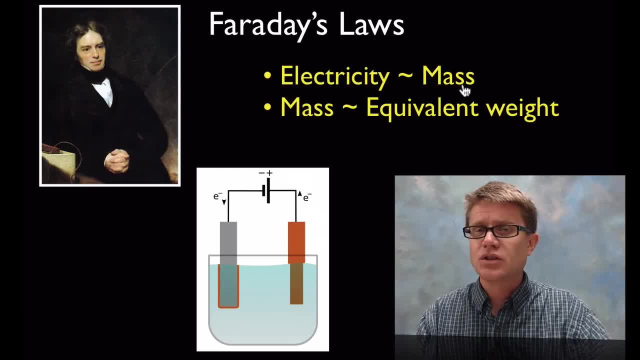 more electricity that we apply to a cell. it's directly related to the amount of mass that a cathode or an anode is going to gain or lose. We also have an equivalence in Faraday's second law to the mass loss is going to be. 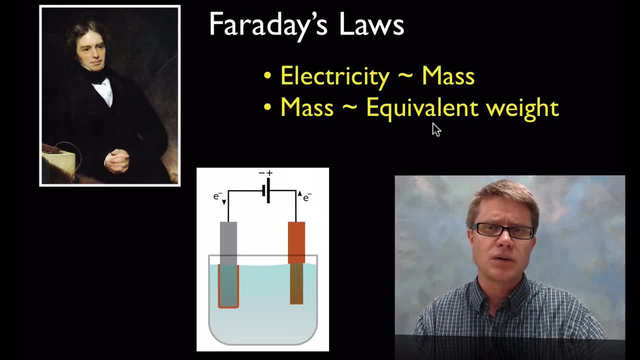 equivalence between the amount of energy that we apply to a cell and the amount of energy that we apply to a cell, And that's equivalent to the equivalent weight of that cathode or anode. What does that mean? Well, if we have something like copper and silver as two of our electrodes, what we would 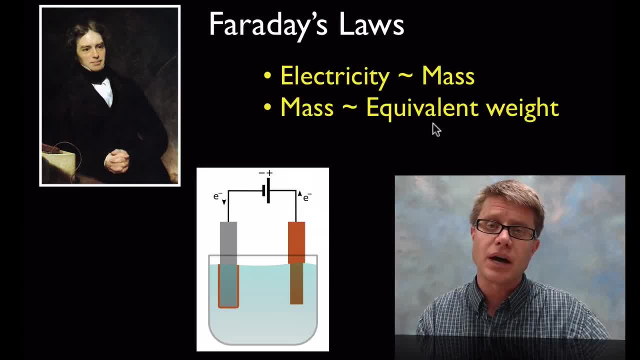 find is that silver, since it has a higher molecular weight, is going to actually lose more mass over time, And so that shouldn't seem surprising if you're looking at it as the losing of atoms from either the anode or the cathode, And so you should have learned. 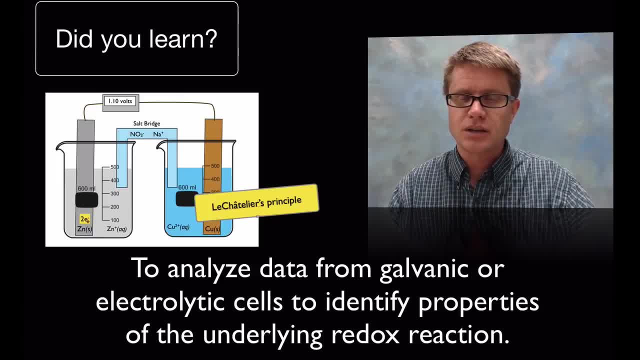 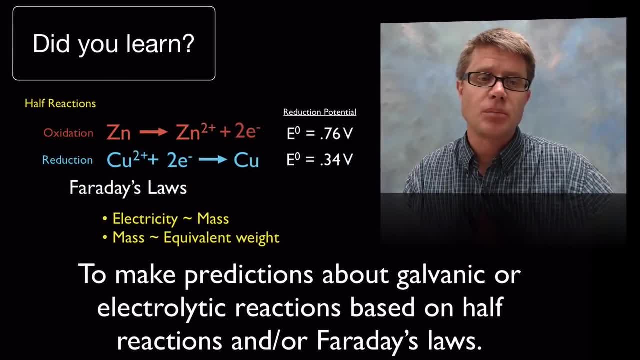 the following: Did you learn to analyze data from galvanic or electrolytic cells? Did you learn to analyze data from galvanic or electrolytic cells? In other words, can you identify what is the reduction port and what is the oxidation part? And then, finally, could you apply half? 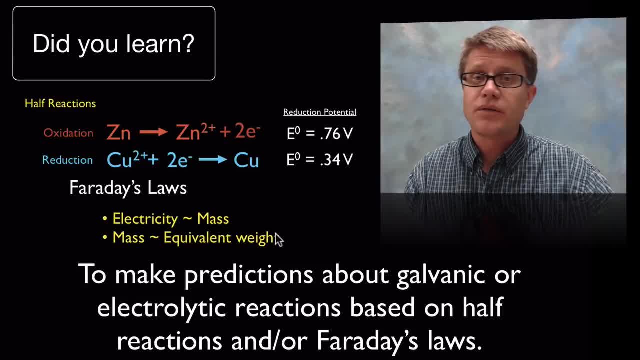 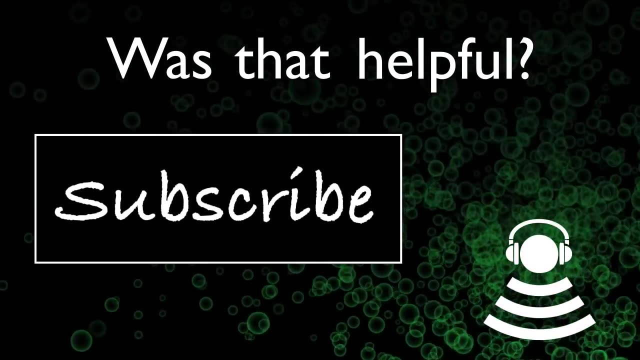 reactions. again, we did that with reduction potential or Faraday's law, to see what's going on in a cell. Well, if you did, you learned what I hoped you would learn, And I hope that was helpful. Thank you very much.